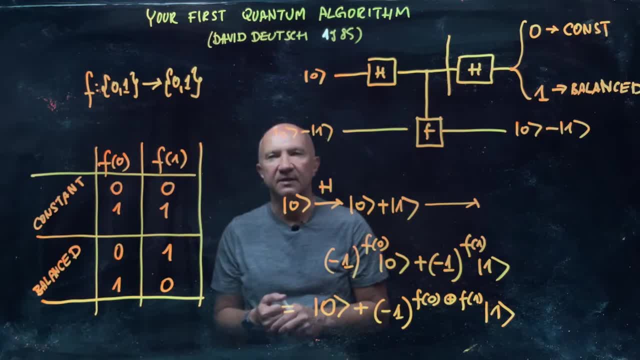 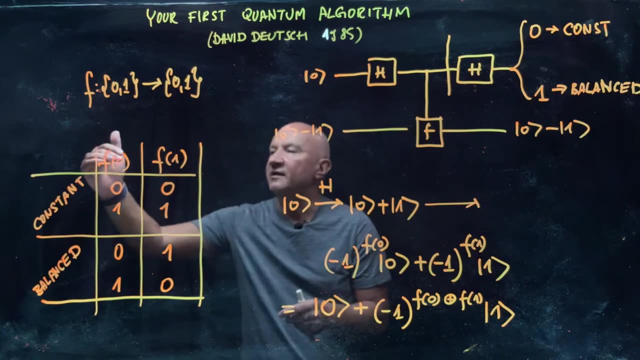 precious box. You run it and it will just cost you money, So you'd better not run it too many times. The problem you have to solve is to tell me whether this black box is evaluating constant or balanced function, And it could be any of the. 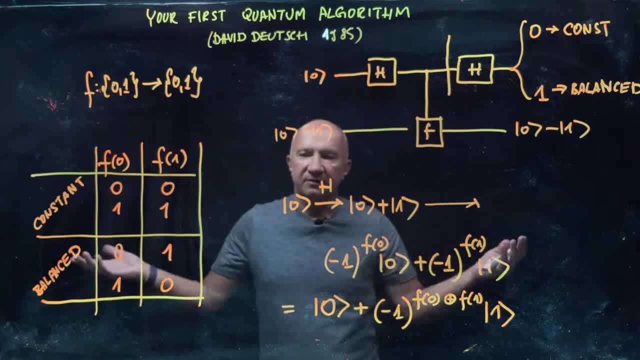 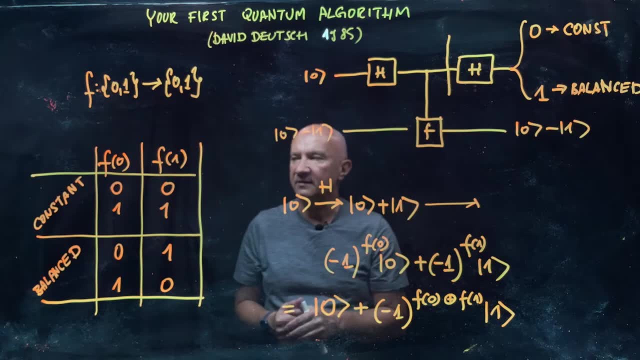 functions. It could be any of the four boxes, right. Then you decide to run it. You have to run it at least once, of course, to get some information about it, And you can see that whatever you get, whatever output you get, it's not going. 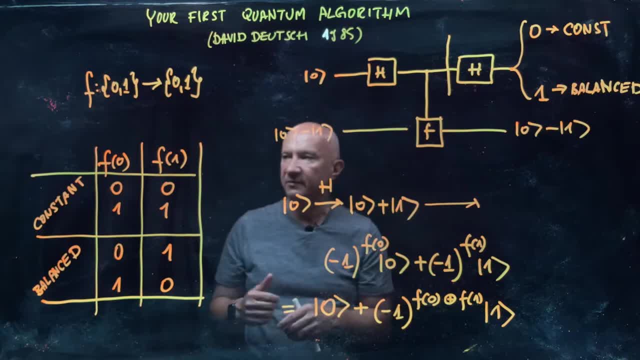 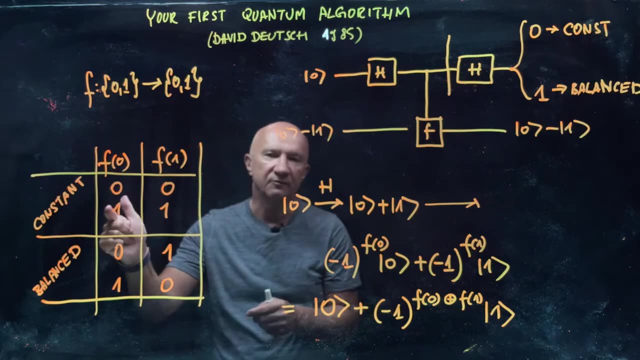 to be enough to answer the question whether it's constant or balanced, right? So suppose you run it on input 0 and you get output 1.. Well then you look at this simple table and you think: well, is it constant at 1?? 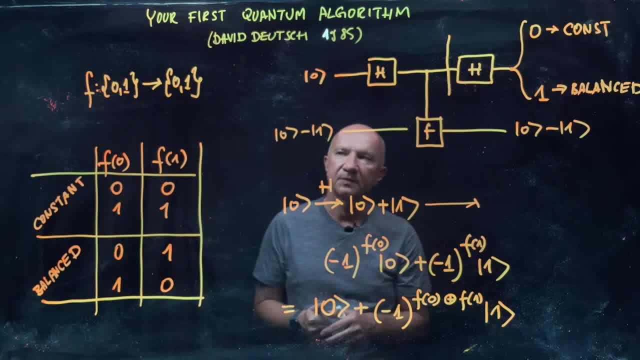 Or perhaps it's just balanced at: f of 0 is equal to 1.. So you have to run it twice, right? So quite clear that in a classical scenario, you have to run it twice to get the answer. In fact, you know running it twice. you are overdoing this because you know exactly which. 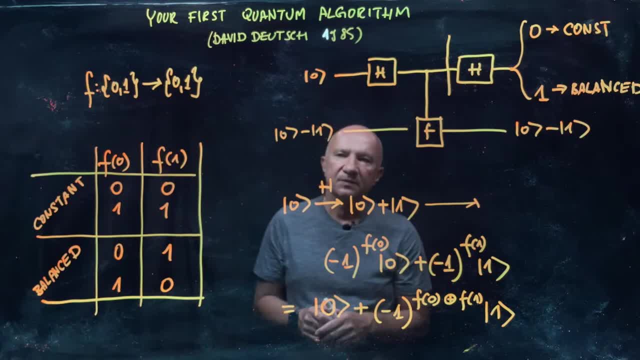 function it is, But so be it. Now, how about the quantum scenario? So here's a slightly modified version of David's solution to the problem. So imagine that you are given this function. You are given this black box, but this time it's a quantum function evaluation which. 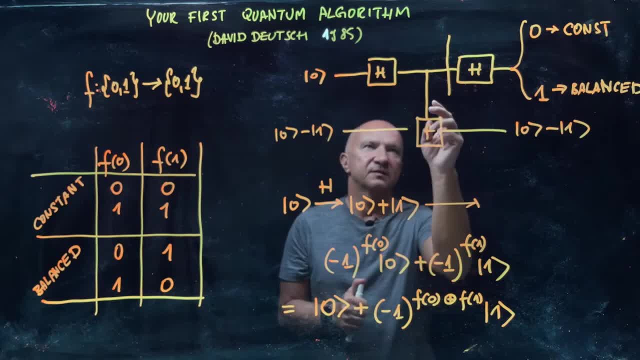 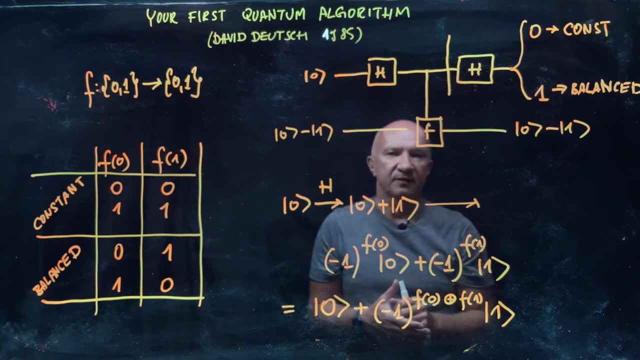 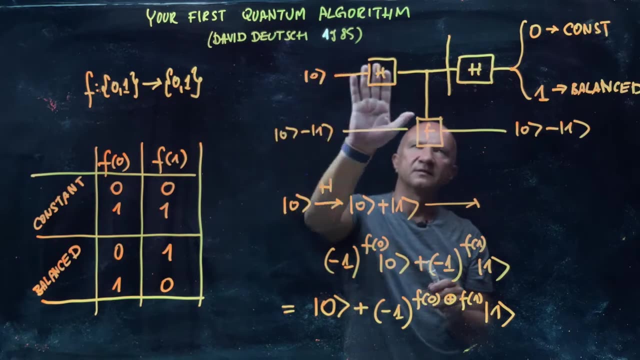 takes input and generates output. So there's this input qubit here and the output qubit would be here, But we sandwich this quantum function evaluation between the two Hadamards here. So if you look at this circuit diagram, here we have two qubits. 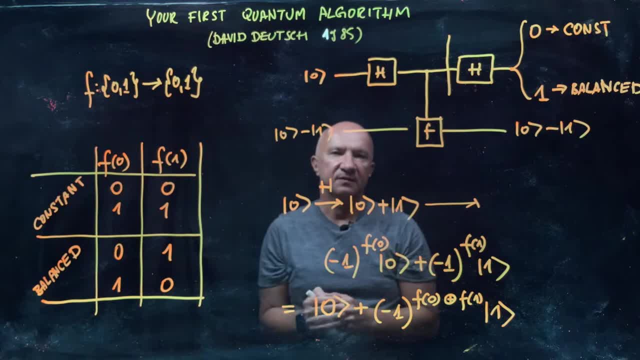 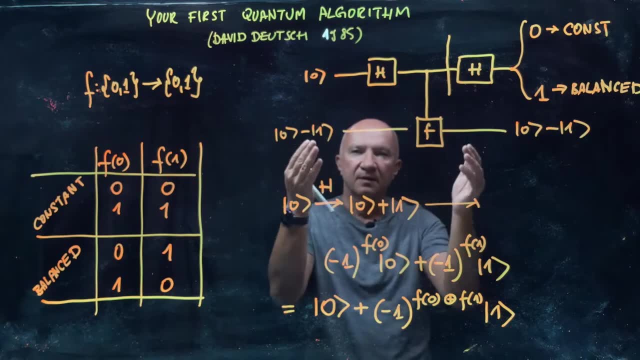 We prepare the first one in state 0.. We prepare the second one in the state 0 minus 1.. So we prepare it in the state 0 minus 1, as you know that we are going to be relying on the phase kickback. 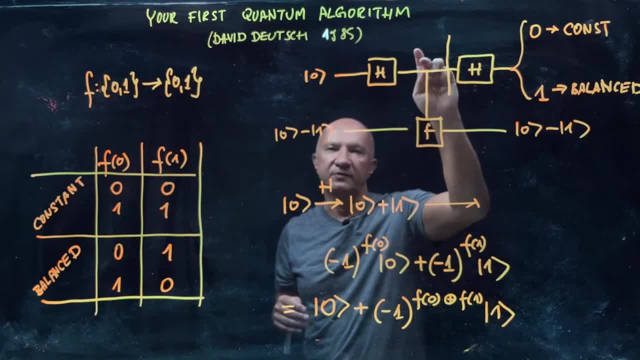 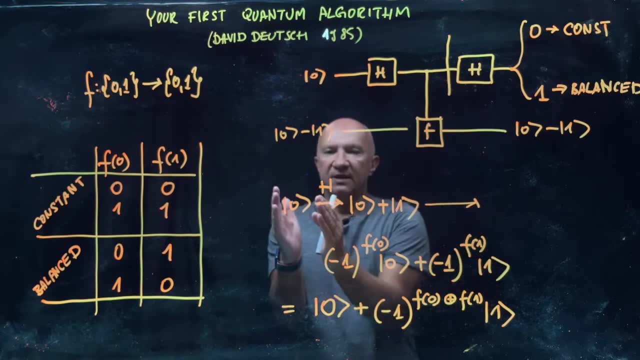 So this black box here will introduce some phase factors here. But let's step through the circuit and see what happens. So we start with the first qubit in state 0., Then the qubit undergoes the Hadamard transfer, So that becomes an equally weighted superposition of 0 plus 1.. 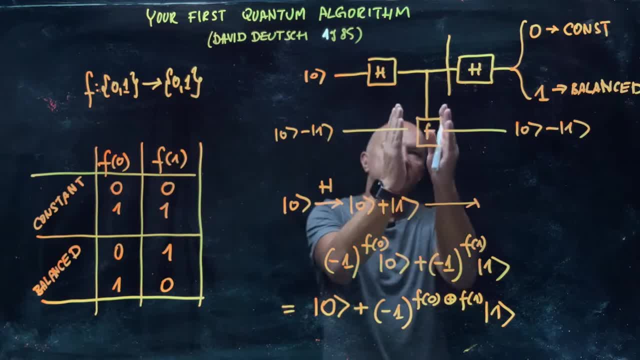 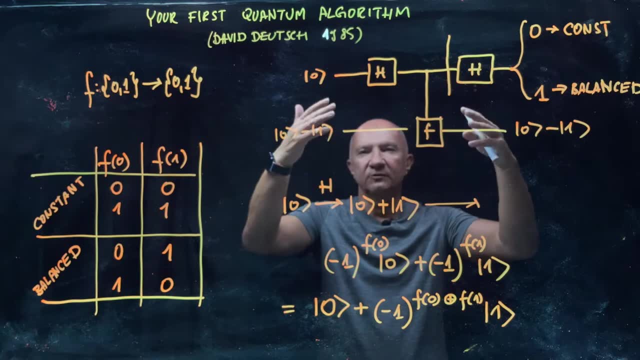 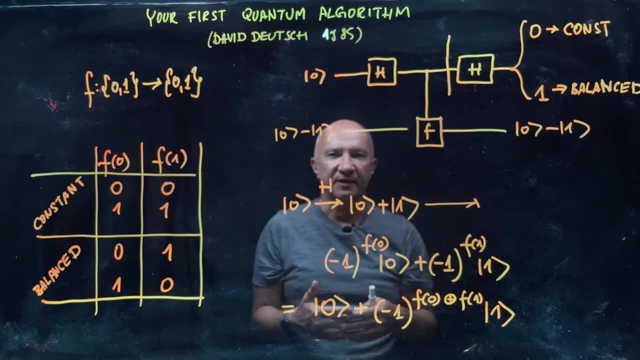 I'm just dropping the 1 over square root of 2.. Now we come to the quantum function evaluation And, as we know, it will not do anything really to the second qubit. but the effect of the quantum function evaluation for this particular oracle is to introduce the phase shifts in. 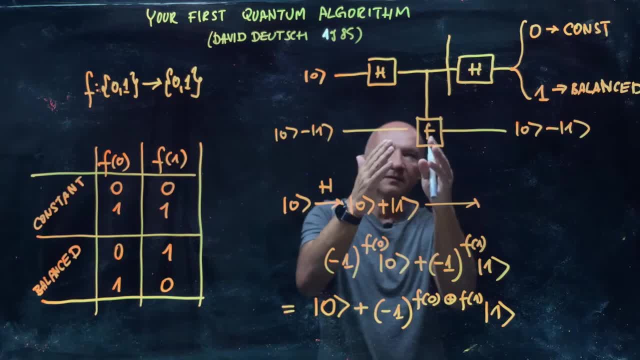 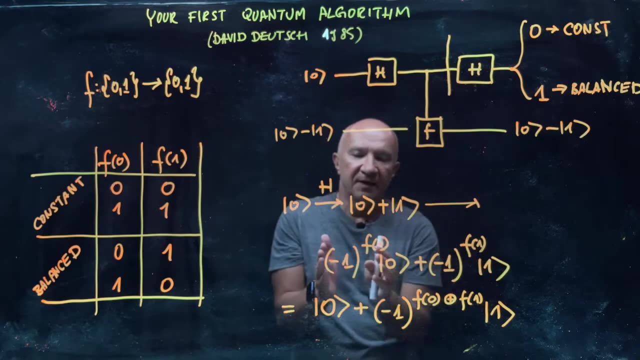 the first qubit. So if you then look at the state right after the function evaluation- the state of the first qubit- the second qubit will just stay in the state 0 minus 1.. So I'm just not tracking the second qubit here. 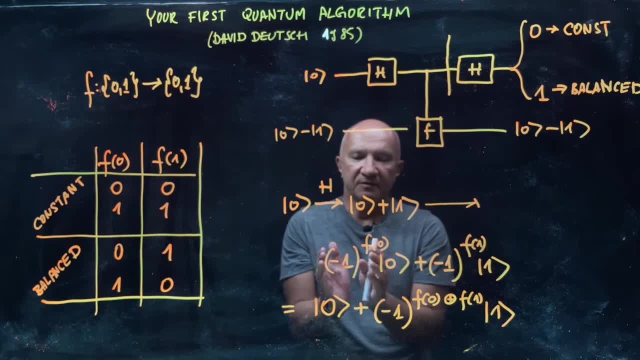 So in this case, after the function evaluation, we will have a phase factor minus 1 to the f of x in front of ket. that represents x. x is equal either 0 or 1.. OK, one in this case. So I have minus one to f of zero in front of zero and minus one to f of one. 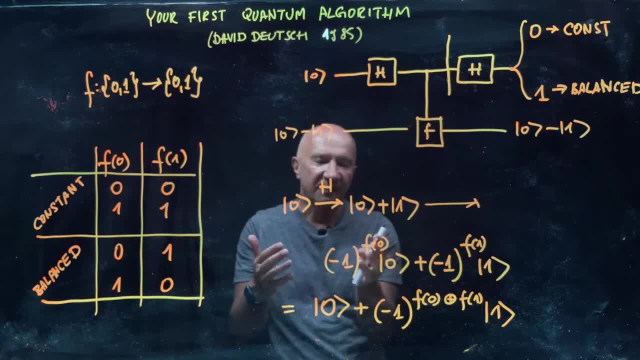 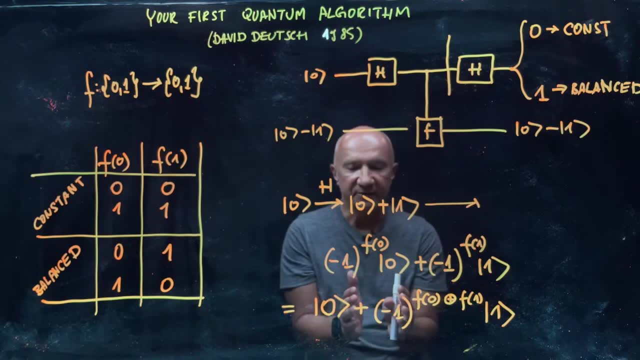 in front of one. So I'll just I factor out minus one to f of zero and then I have a state with a relative phase, because that's really what matters- And, as you can see, this is equal to this phase. factor here is minus one, f of zero plus f of one. So we have here the binary addition. 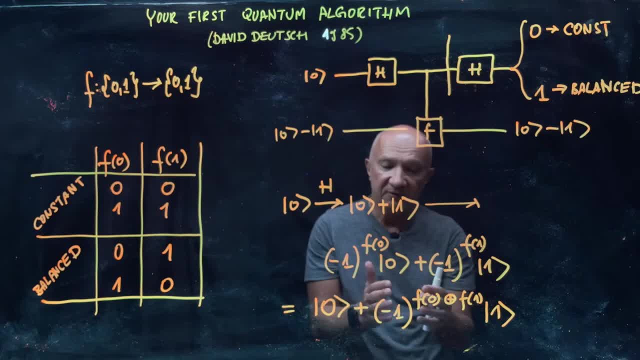 f of zero plus f of one. So the phase factor is either minus one or plus one. So here I have either state zero plus one or zero minus one. When? So when this? when the two values of the function are identical. So if the function is constant, so the f of zero plus f of one in this, 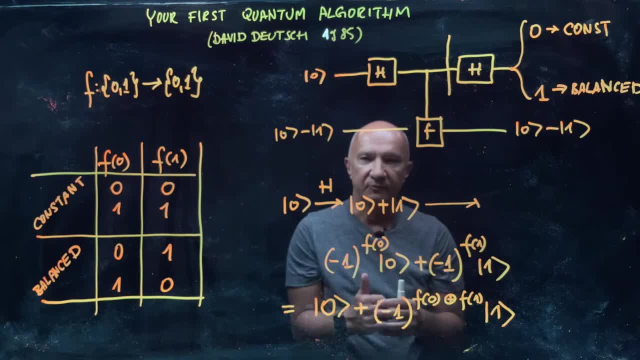 case will give me zero. So this phase factor will be plus one. So therefore I will have a state zero plus one, Which will then, after the second Hadamard, give me output zero. So when I see the output zero, I know that the function is constant. Now, if the two values are different, then f of zero plus f.